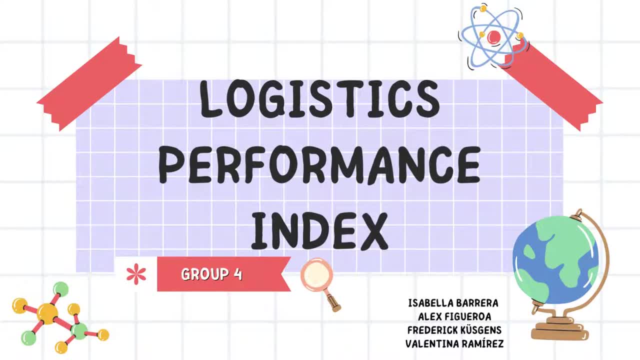 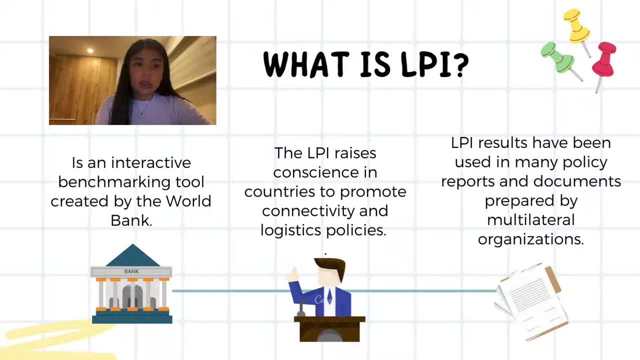 What is LPI? The Logistic Performance Index is an interactive benchmarking tool created by the World Bank to help countries identify different challenges and opportunities they face in their trade logistic performance and what they can do to improve their performance. So the LPI raises consciousness in countries to improve connectivity and logistic policies. 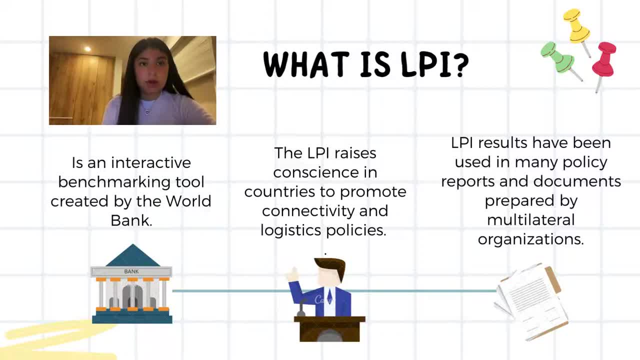 It is not considered a diagnostic tool, but rather a general metric on the efficiency of supply chains, So a data collection is carried out where there are a number of countries survive. For example, in 2018, there were 160.. the responders rate their country and eight other countries, and 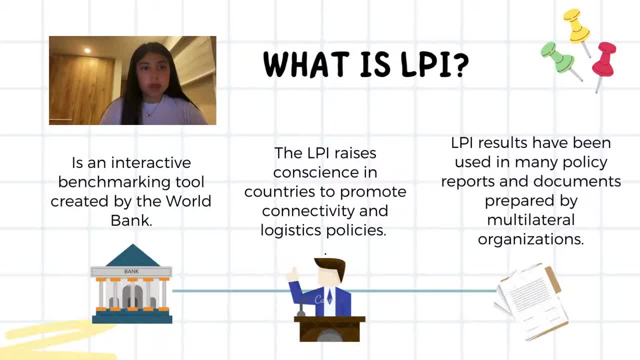 six components are: rate on a scale of one to five, Customs, infrastructure, quality of service time, international achievements and traceability. So this course of the six variables are add to a single value using principal component analysis, PCA. The output values. of the PCA is a single indicator Which is the average weighted value of all scores. 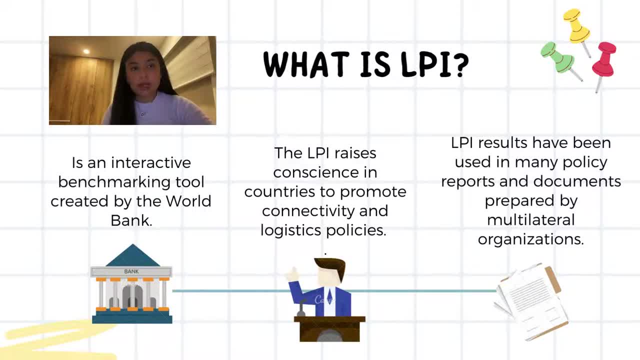 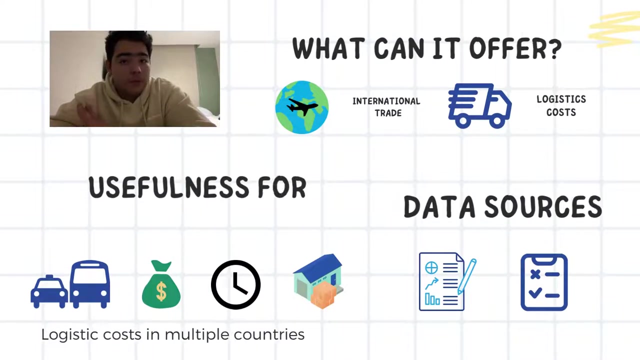 And finally, LPI results have been used in many policy reports and different documents prepared by multilateral organizations, and findings from the index provide a worldwide General benchmark for the logistic industry and for logistic users. LPI is a tool used by multiple companies around the globe. This is able to measure logistic costs around the globe. 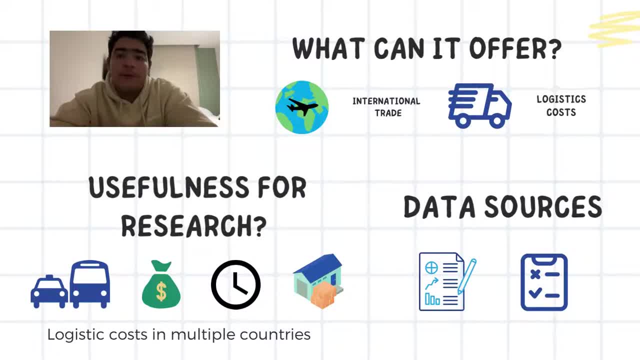 as well. this has helped companies to make deals around the world by facilitating the international trade. The tool is able to measure logistics costs on any country and improves companies efficiency with this. LPI provides information of transportation cost, shipping time, warehouse costs and picking accuracy on any country as well by helping with custom procedures on. 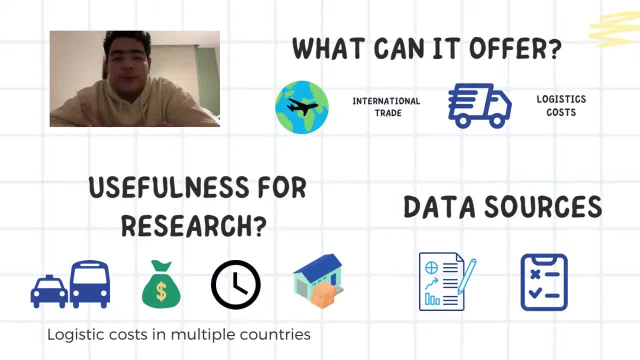 Maritime and overland infrastructures. LPI Commonly uses monthly and annual data Recollected through surveys that states how logistic costs are behaving in multiple places at the same time around the world. in order for surveys to work, Local companies and independent workers are the ones in charge of filling them up with all the information. the LPI 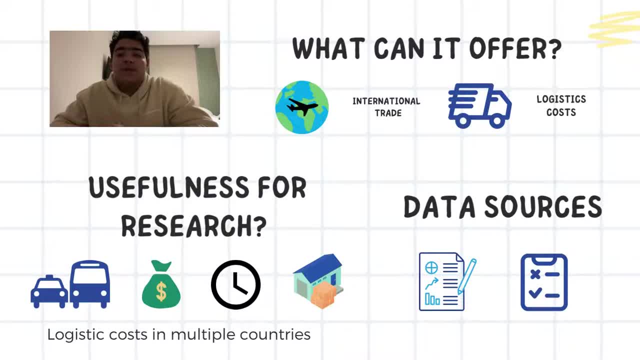 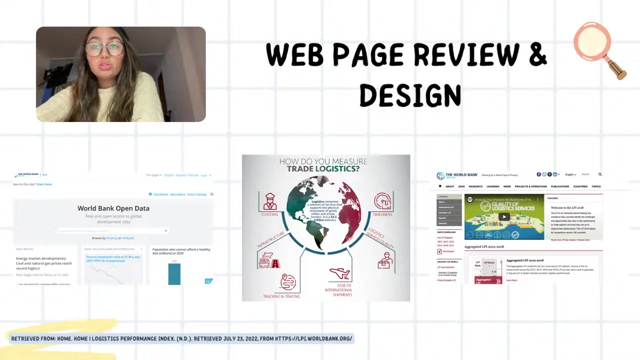 tool requires. This is to work efficiency and also by working with the World Bank database, They are able to provide to their customers a real data time, a real-time data to make international trade much easier. The World Bank website has multiple information resources about the processes, solutions and services. 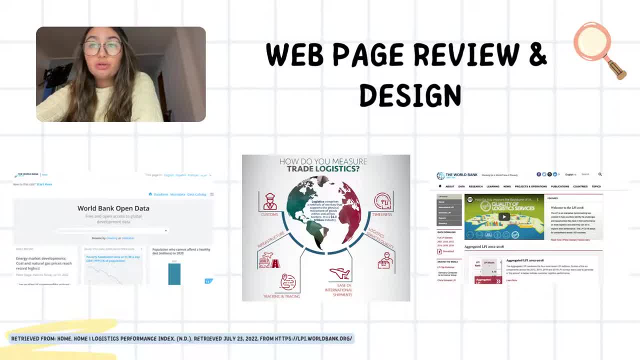 They offer to countries for improving their LPI performance. In this website, information about who the World Bank is, the mission they have, on the projects They lead is given, Emphasizing on working for a world free of poverty- mantra They work on every day. it offers hyperlinks where countries can find yearly LPI reports and comparisons about it. 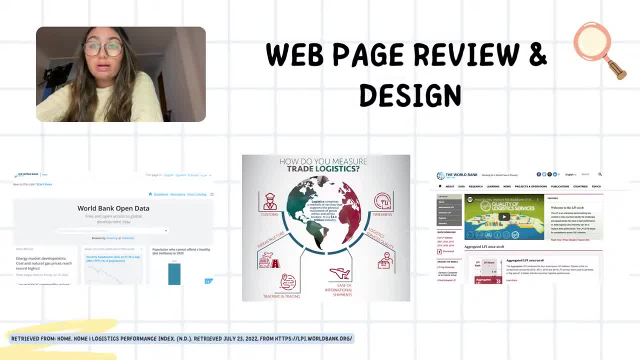 the news section emphasizes on humanitarian crisis, economic development and the pandemic impacts around the globe, as well as Informative flyers can be found throughout the website in order to inform countries about their logistics Operations, how to improve them and keep them up to date about the outside world's behavioral process. 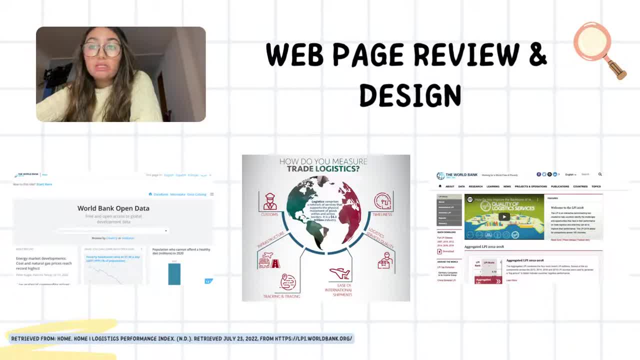 something that is important to note about the World Bank's website is that it has a Specific section where you can search for anything about a country, and the results will be supported with graphics for a better understanding. It can also be said that This web page is very complete, since it has a very valuable information for the improvement of the internal 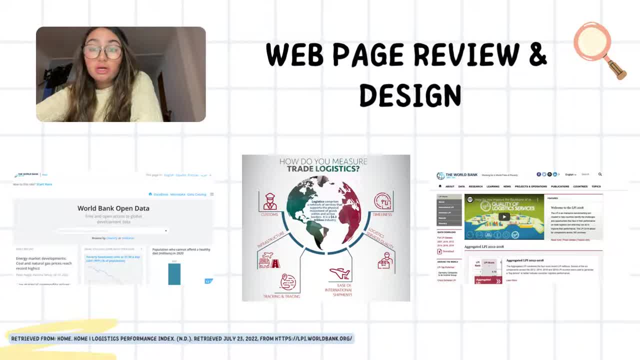 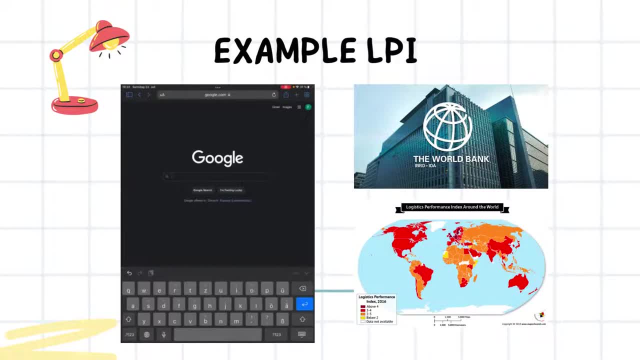 logistics processes of each country, better known as LPI, As the API can be an important KPI for companies. it can help companies, for example, to select suppliers or business partners. The World Bank provides the list of APIs of the different countries online. You can simply Google, have it like. 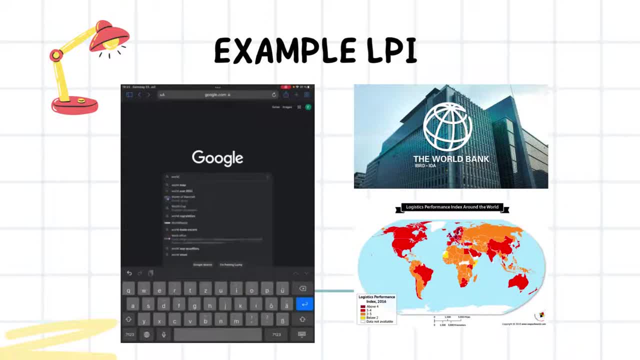 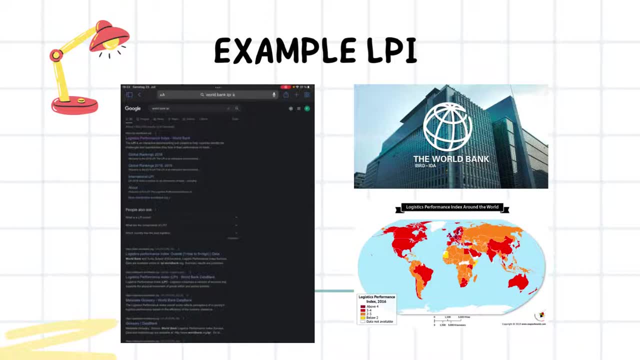 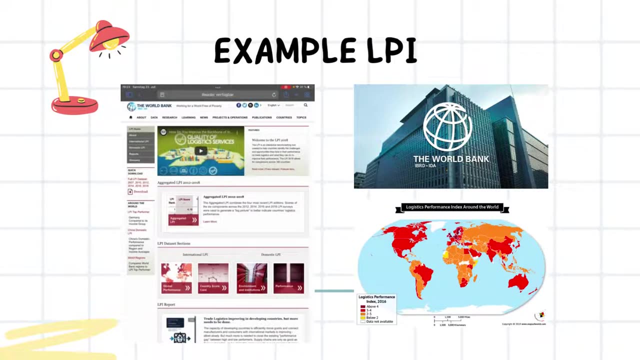 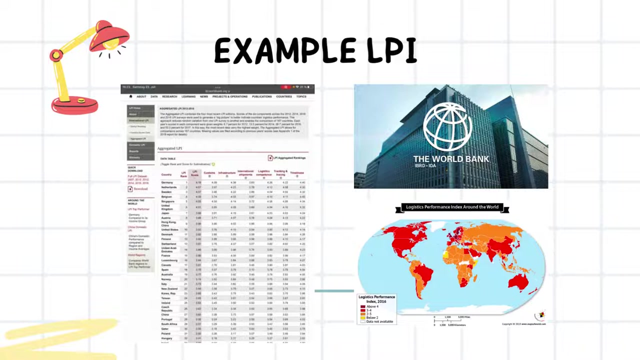 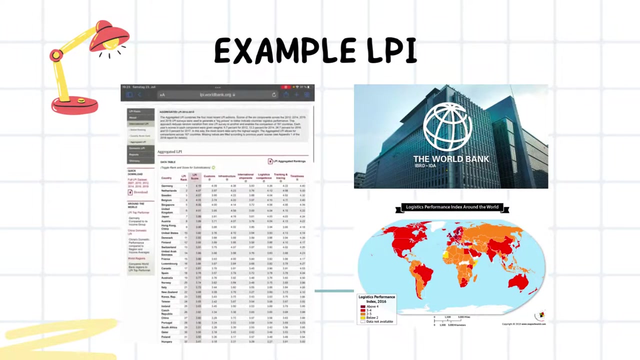 World Bank Where undo, Bank, AO, SEO and You can go on the first page on logistics performance index from the World Bank. CHOICE đây the LPI score. there are almost all countries in the list. more precisely, there are like 167 countries, as you can see here at the top and, yeah, the LPI. 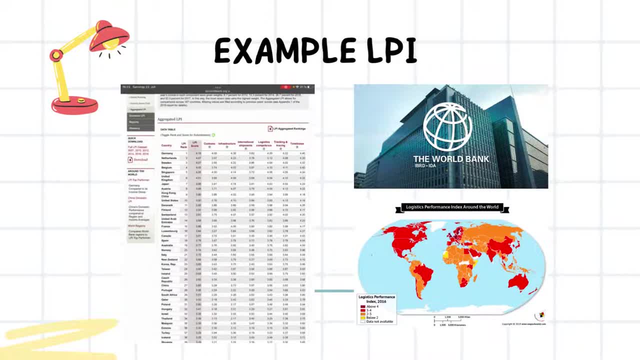 score is an average score from the years to from 2012 to 2018, and the LPI score is composed of several factors, like you can see here: infrastructure or international shipments, and the LPI can be used when a company got different, for example, when a company 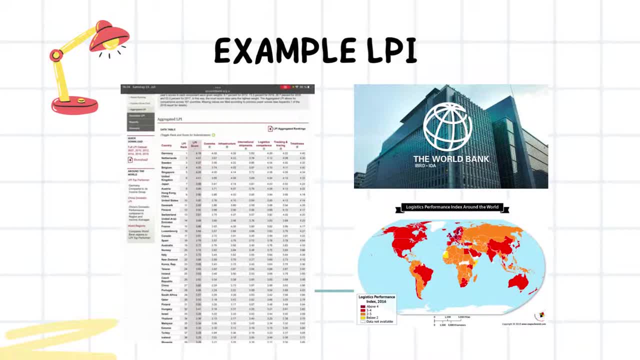 got different offers from suppliers out of different countries and the price and the other condition are quite similar, then the company can compare the different countries with the help of the LPI, for example, one offers from a supplier in Belgium and one offers from a supplier from Poland, and then you can. 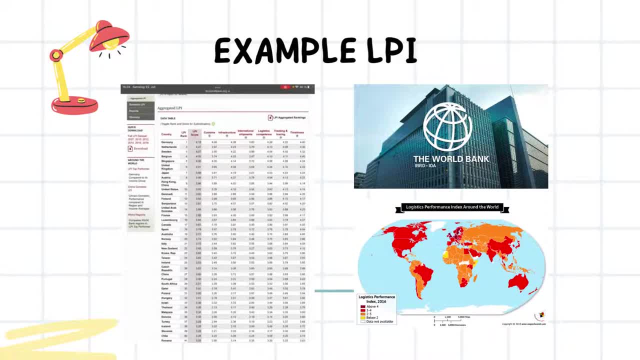 compare the both both countries and you can see that Belgium has a better API score. so the companies hold, then choose the offer from the supplier from Belgium because Belgium has a better API score and a good API can reduce the risk of delivery failure, for example due to a poor infrastructure, and you can see that.